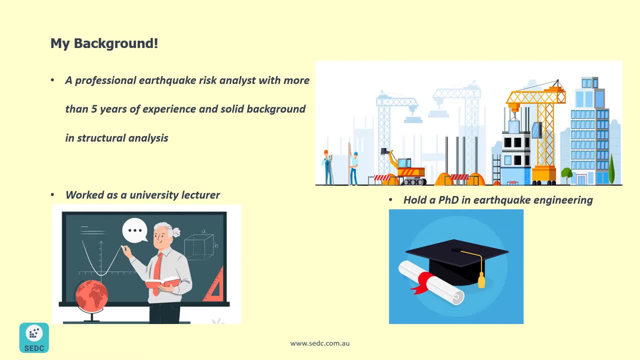 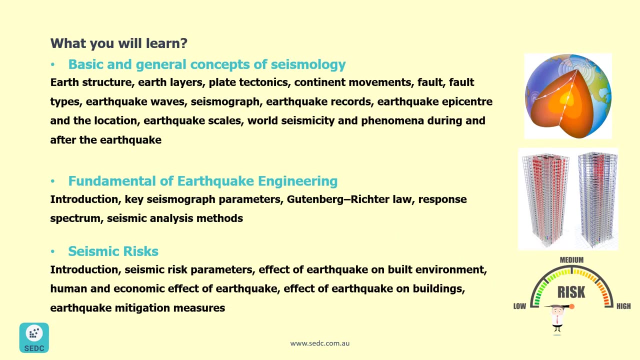 than thousand students. I've created this course to give you the skill and knowledge to be prepared for the earthquake, engineering design and make yourself familiar with the fundamental of the seismic behavior of the structures. In this course, I will talk about some of the basic concepts of seismology which I 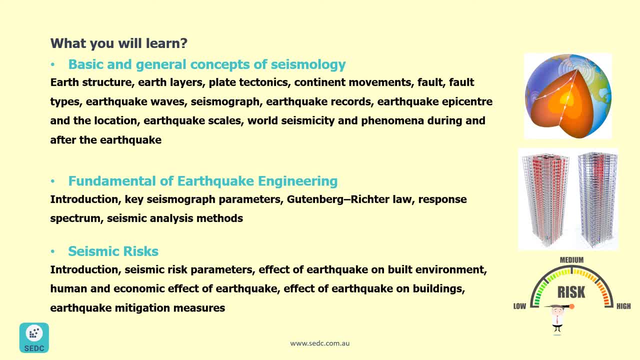 learned in this course. My general approach in this course is to explain some basics and general concept of seismology, followed by earthquake engineering and risks. So in the first section, which is seismology, I will cover earth structure, earth layer plate, tectonic continent movement, fault and fault types. 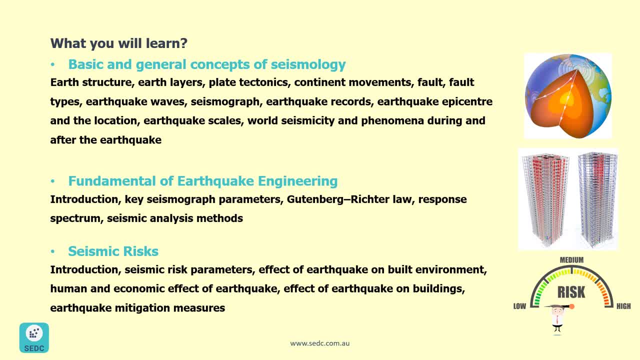 earthquake waves: seismograph applications, earthquake scales, world seismicity and, finally, phenomena during and after the earthquake. In the next section, which is earthquake engineering, I will give you a little bit of introduction and we'll talk about the key seismograph parameters. Gutenberg-Richter law. 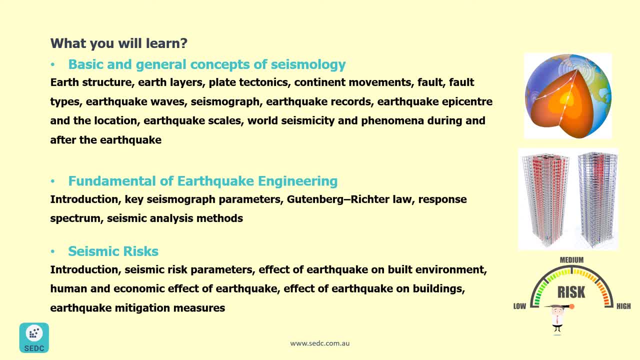 response: spectrum and seismic analysis methods. In the last section we will cover all the seismic risk parameters, for example, seismic risk, seismic risk estimation, seismic risk analysis methods like static analysis, seismic risk analysis methods, static analysis, spectrum analysis and time history analysis. 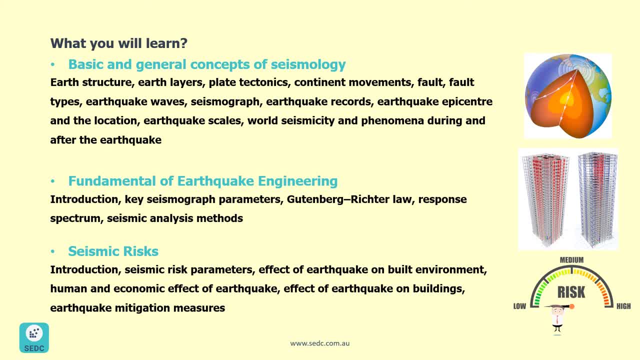 Finally, in the seismic risk section, we will have again a little bit of introduction, talking about the seismic risk parameter, effect of earthquake on the built environment and the building, human and economic effect of earthquake and, finally, earthquake mitigation measures. This course is beneficial to everyone who is interested in it and knows how to use it. I really encourage you to check out the course. 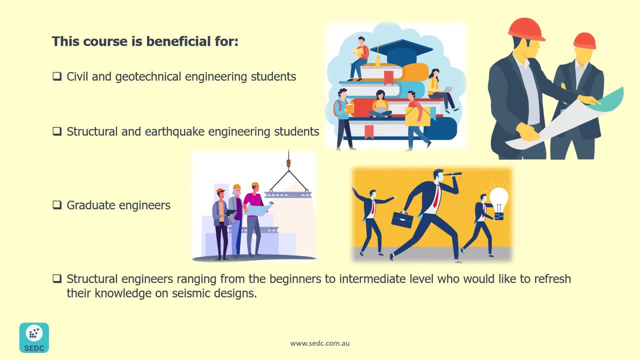 all for civil and geotechnical engineering students, structural and earthquake engineering students, graduate engineers and structural engineers, ranging from the beginners to intermediate level, who would like to refresh their knowledge on seismic designs. by the end of this course, you will learn about the fundamental and detailed mechanism of the earthquake and seismic design.